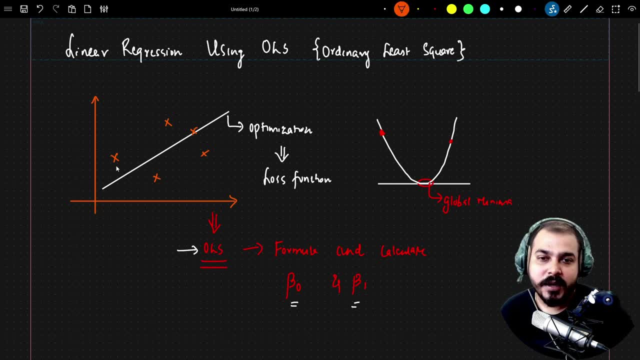 Again, as usual, the aim of ordinary least square is that we should try to reduce this error, right? We should try to reduce this error that is, between the predicted and the truth point, right. So this is basically the error with respect to any best fit line that we create, right. 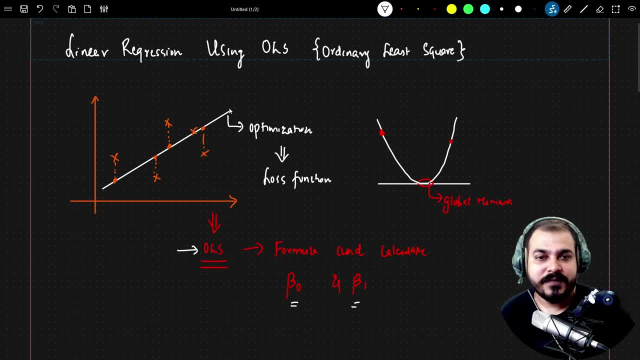 So here, what you can do is that again, let's say that if I have another line, if I have some line like this, So for this the intercept will be different, the coefficient will be different. For this, the intercept will be different, the coefficient will be different. 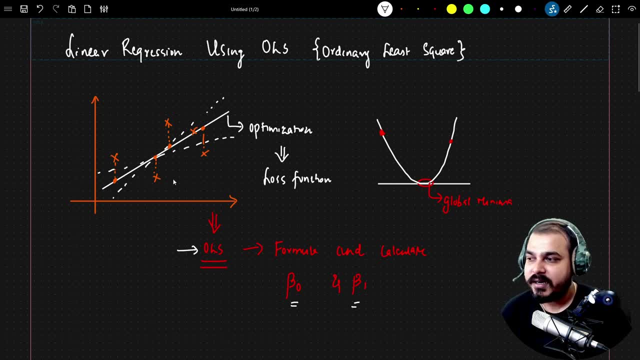 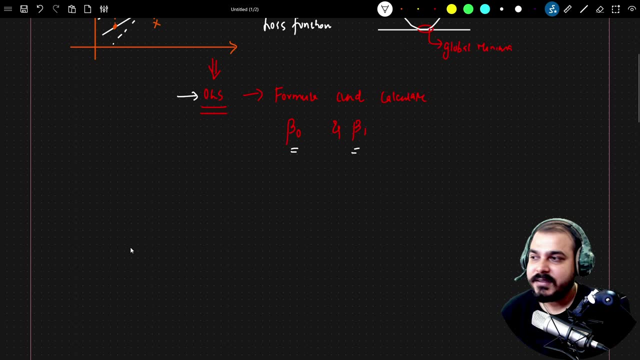 But we should try to select that line which gives us a less error. So, So, So now let's go ahead and let's try to derive the formula for OLS And again, guys, OLS. here I'm just going to give a notation. 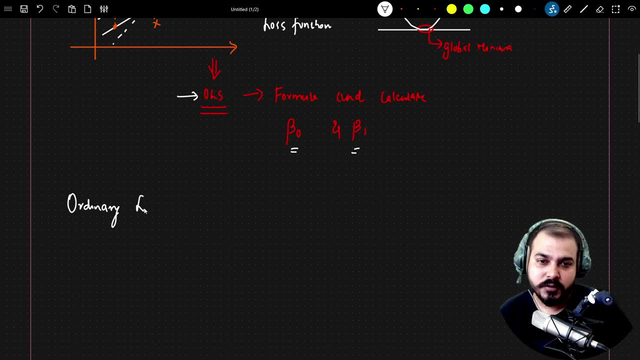 Let's say this is my ordinary least square. okay, You know what is the aim of ordinary least square? I'm going to give you a notation. with S Let's say this is beta zero and beta one. Let's consider that this best fit line is given by h. theta of x is equal to beta zero. 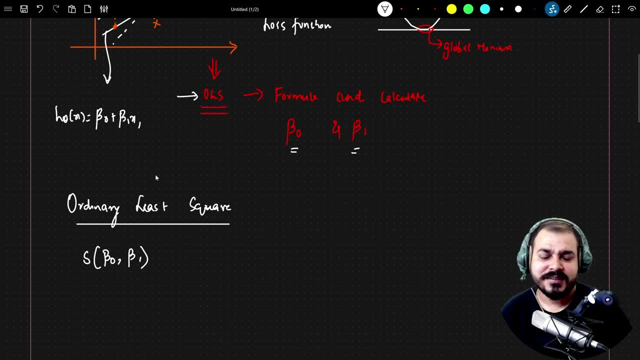 plus beta one into x one. I'm just considering this as a simple linear regression And I said in the ordinary least square. I'm not going to use any loss function like mean squared error, but I'm just trying to say that, okay, I have a scenario wherein I need 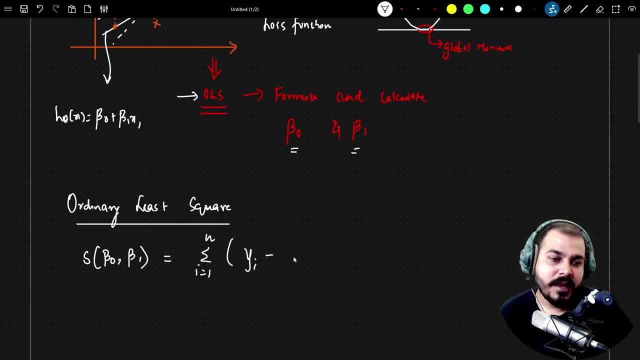 to reduce my difference between y of i and h theta of x. What is h theta of x? h theta of x is nothing but beta zero plus beta one multiplied by x one. And this is nothing but my predicted value y hat. So I'm just going to use this: 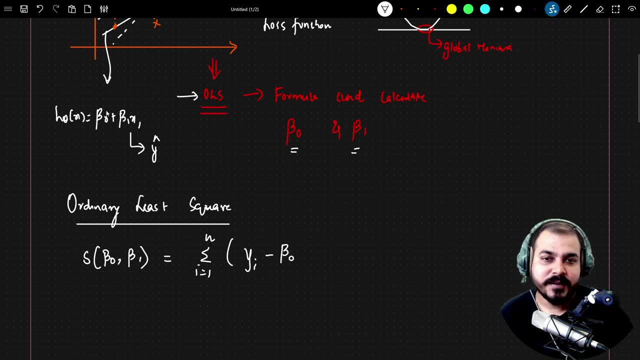 Okay, So I'm going to use this particular equation like this and probably write over here: This minus will get subtracted to this, okay, So it will become minus beta zero, and it will be minus beta one into x one, And this should be whole square. 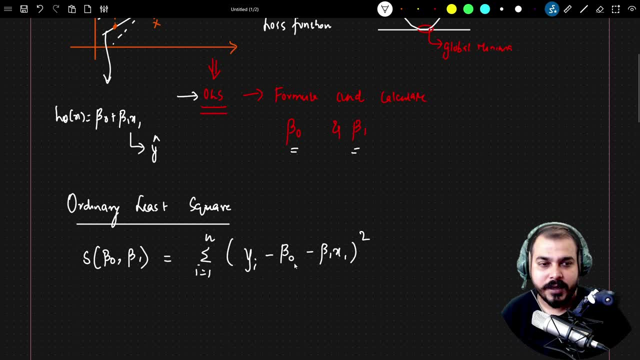 So here, what I'm doing is that I'm just trying to reduce the error, okay. My aim is that this difference that I'm actually getting this is basically the error, okay, And I'm just going to reduce this specific error and obviously this basically looks like: 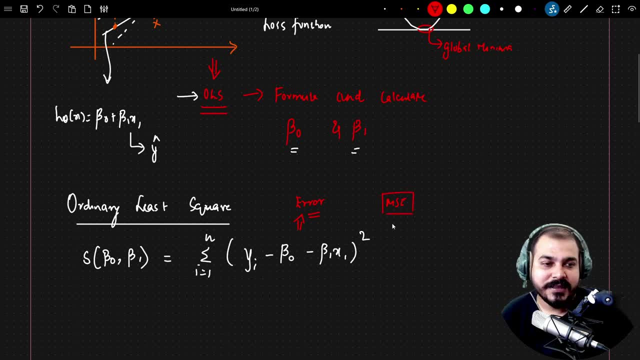 a mean squared error formula itself, right. So OLS by default. I think it uses mean squared error, okay, And if I try to find out the average, it will be divided by n, okay, So one by n multiplied by this. 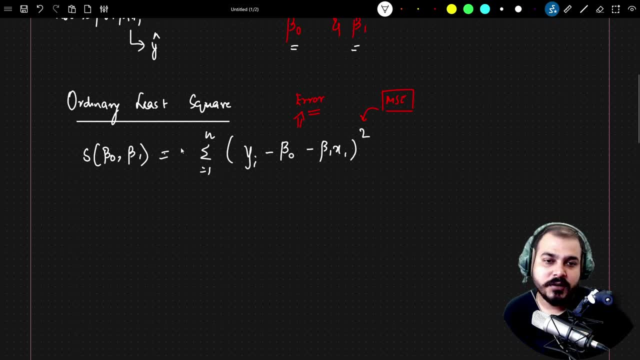 So here let me write it by white pen only, otherwise you'll get confused. So this will be one by n, y of i minus beta zero, plus beta one into x one, Now in ordinary least squares. the aim is we need to calculate beta zero and beta one. 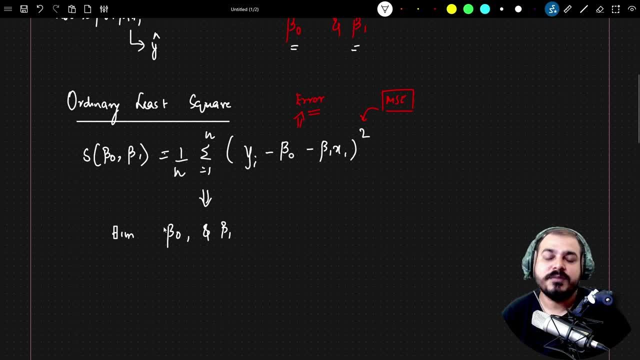 okay, And obviously we'll try to derive the formula through which beta zero and beta one can be calculated. So before I go ahead and talk about this, you know, in gradient descent also, we try to find out derivative right with respect to every coefficient and we try to come to 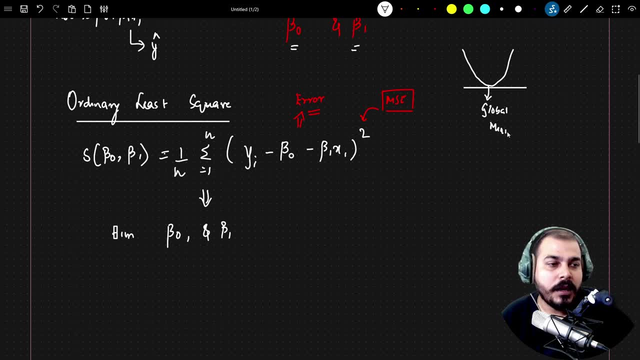 the global minimum. okay, Now, what we are trying to do is that we are trying to find out what should be the formula of beta zero and beta one. In order to find it, first of all, what I'll do is that I will try to calculate the derivative. 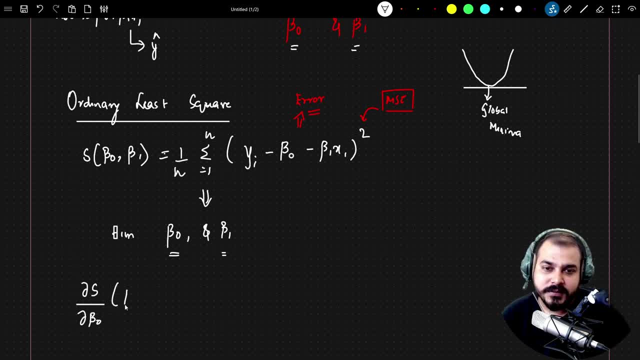 So derivative of ds of d, beta zero. Okay, And let's say beta zero, comma, beta one is over here. Here I can specifically write this as okay. Now, if I try to find out the derivative of this value, what it will happen, see, guys. 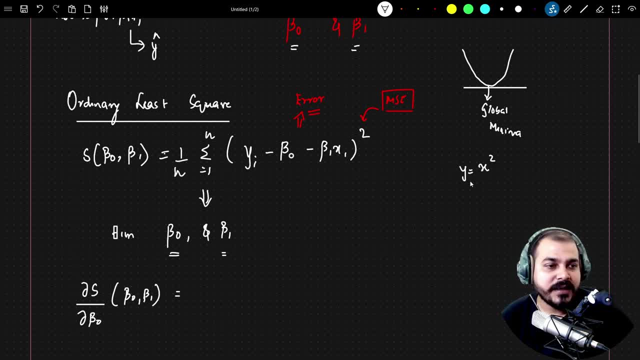 if I have an x square value and if I have y is equal to x square, and if I write derivative of y with respect to derivative of x, then this what will happen: It will say two x two minus one multiplied by x. right. 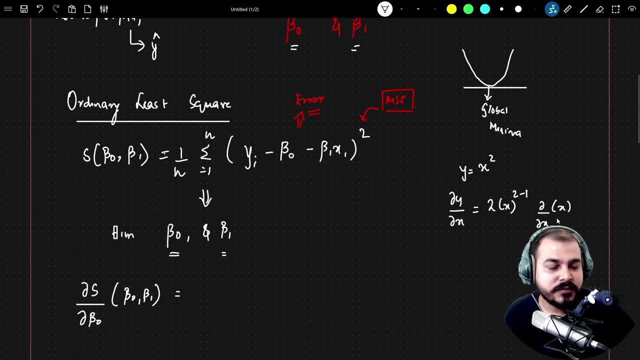 Sorry, It will say derivative of x, right? This is what exactly happens, right? And then, finally, I get two x, because derivative of x with respect to x is one, right? So if I try to, if I have equation y is equal to x square, and if I try to find out the derivative, 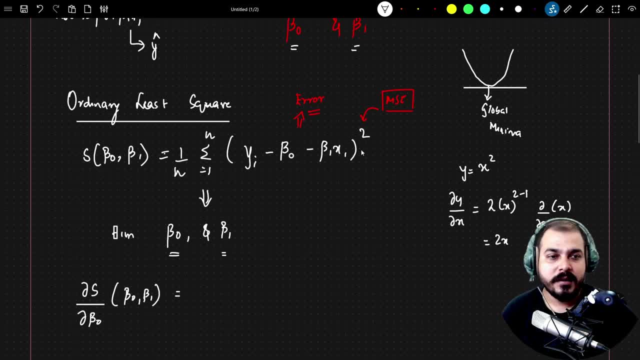 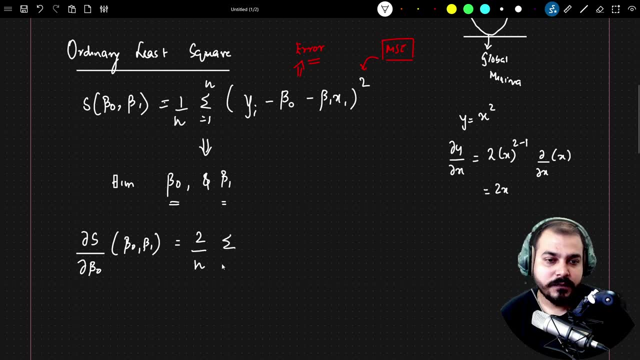 of y with respect to x. I'm going to get two x Now. similarly, over here, you'll be able to see that if I try to find out the derivative, what will happen? This will be two by n. okay, Summation of one to n. 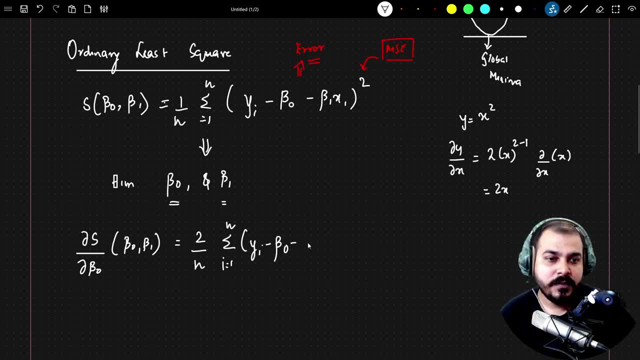 And then I will write. I'm going to write this entire equation y of i minus beta zero, minus beta one x one. Now here it will be two minus one, right, Two minus one. So I'm not going to write one separately over here. 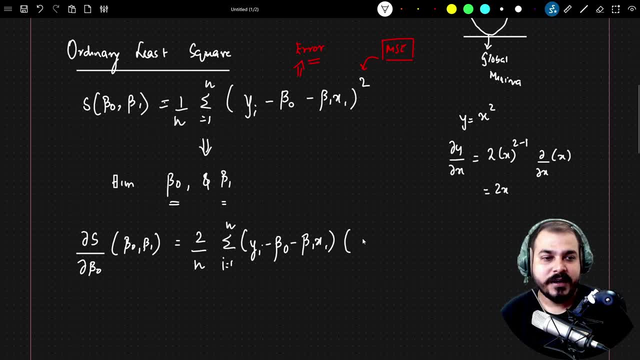 And in the next one I'm just going to find out the derivative of this entire value, right, With respect to beta zero, This becomes a constant. So obviously this will be zero minus beta zero is there. Then this will become minus one. sorry one, because derivative of beta zero with respect. 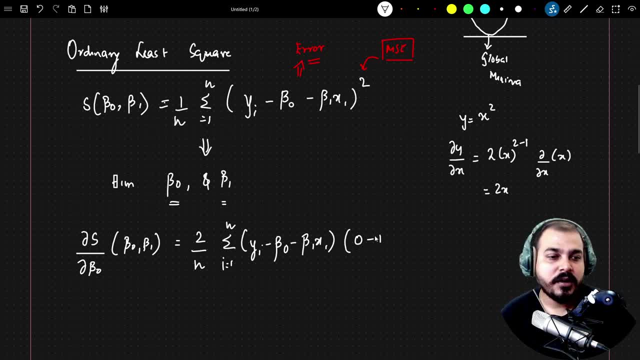 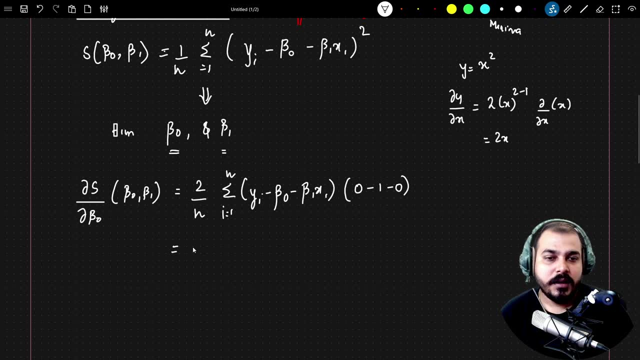 to beta zero is one. And then here you can see that this will again be a constant. so I'm going to write minus zero. So at all. if I try to find out derivative of s with respect to derivative of beta zero with respect to beta zero, comma beta one, I'm going to get two by n minus two by n. 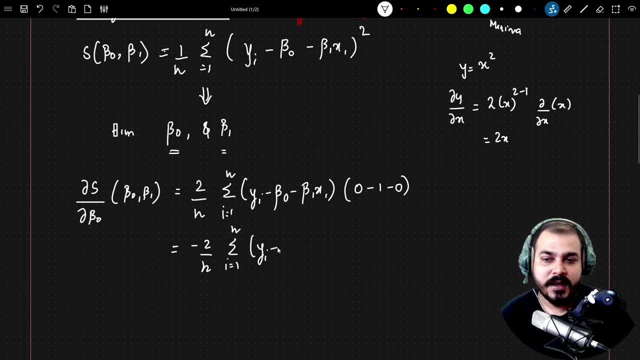 Summation of i is equal to one to n y of i minus beta, zero. minus beta one x, one right. This is what I'm actually going to get. So this I'll be assigning it to zero. So this will become my x. 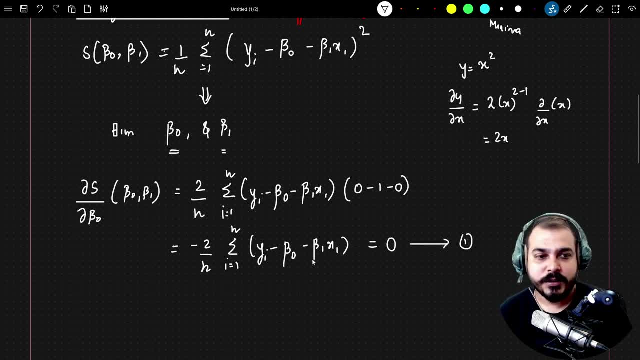 This will become my first equation. let's say, okay, This will become my first equation, because I need to derive beta zero and beta one. Similarly, if I write derivative of s with respect to derivative of beta one, with beta zero, comma, beta one, here the equation that I'm actually going to use, again what I'm 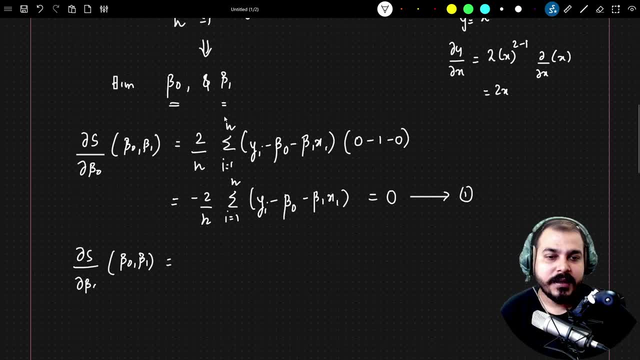 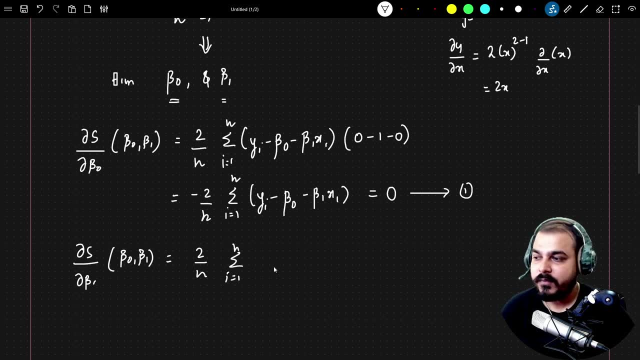 going to do. I'm going to find out the derivative with respect to beta one, right? Then again, it'll be what two by n- okay, And this will be summation of i is equal to one to n, And here I will write y of i minus two by n. 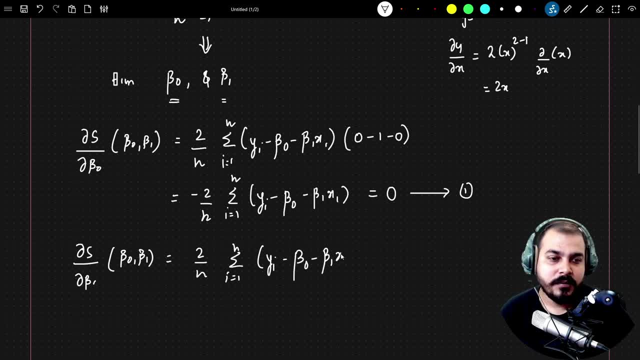 Okay, Minus beta zero, minus beta one x one. Now this entire thing. I have to find out the derivative. Now, this will become a constant, this will become a constant and finally, I'll be getting minus beta one. sorry, minus x one, right. 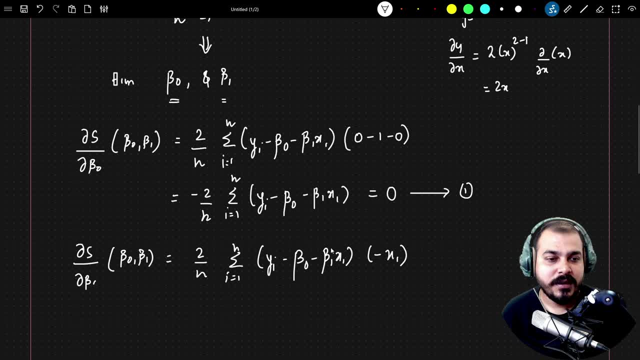 Why x one? Because derivative of this value with respect to beta one, this beta one will become one and x one will get remained right Now, I will assign this to zero. So this will basically become my second equation. okay, And this equation again, I can basically write it over here. 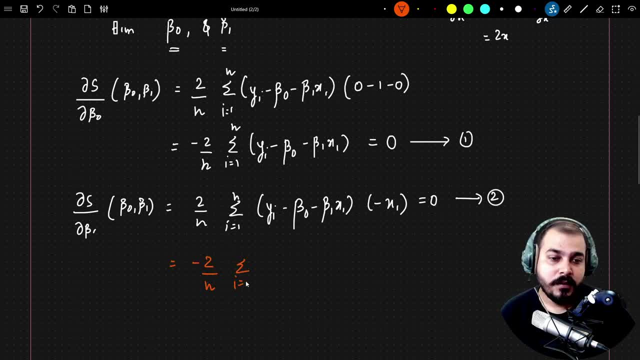 Because I'm just trying to prove you what is the formula. okay, i is equal to one to n beta, zero, beta, one x one multiplied by x one, which is equal to zero. okay, So this is my entire equation and this becomes my second equation. 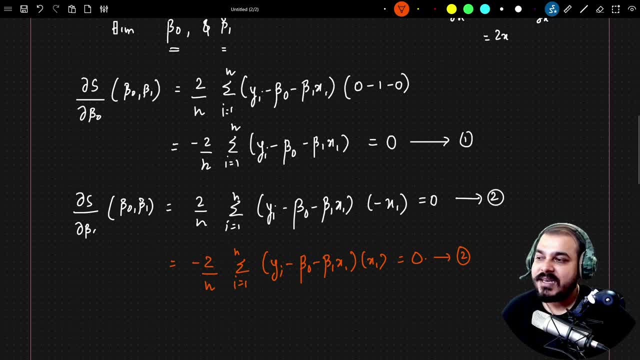 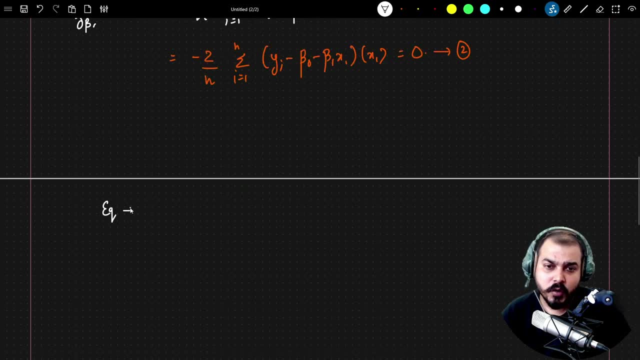 Now, with the help of this two equation, what I'm actually going to do? I'm going to basically simplify this equation and try to find out what is beta zero and beta one, and we'll try to calculate. Now let's go ahead and take the equation one. okay, 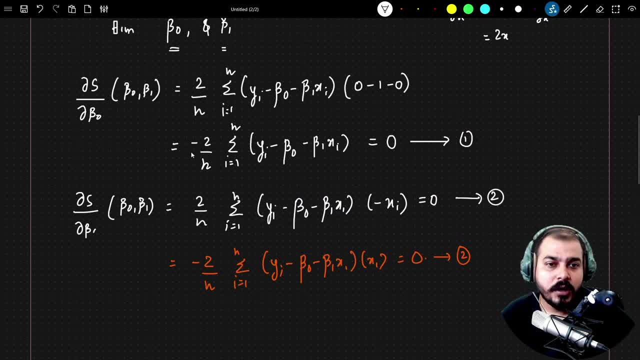 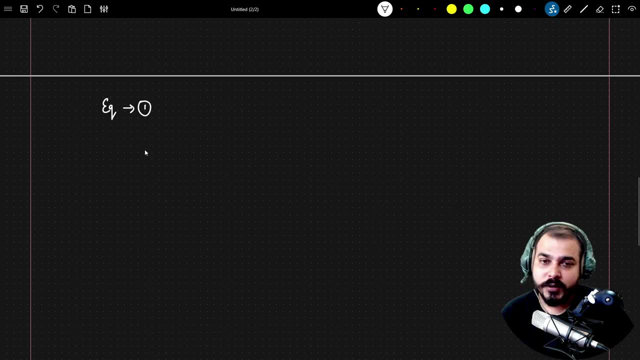 Okay. Okay Now. equation one is what? Two by n right, Minus two by n, summation of i is equal to one to n y of i. minus beta, zero, minus beta, one x one right. So here I'm going to take: minus two by n, summation of i is equal to one to n. 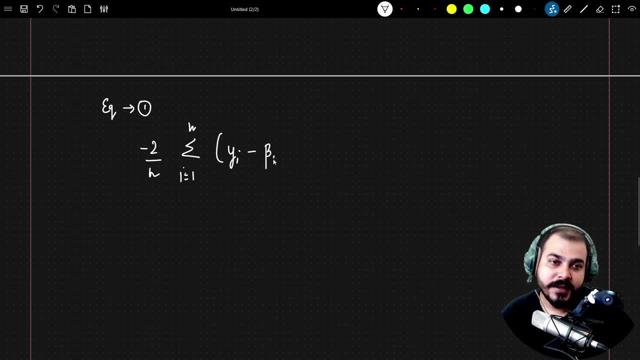 This is y of i minus beta zero minus beta one into x of i is equal to zero. okay, Now let's consider this two. I'm just taking this equation- This is my equation one, and we'll try to calculate what beta zero or beta one will be okay. 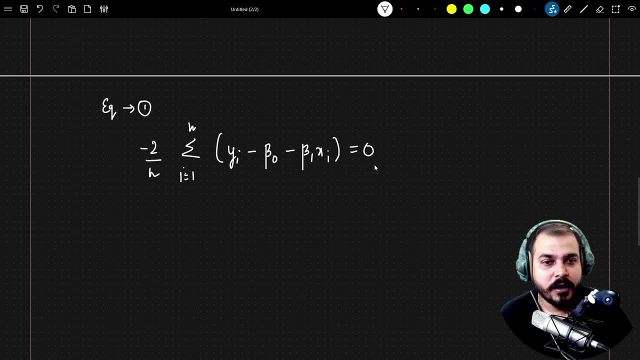 Now, in this equation, when I take this two below and if I put it to the denominator, this will be zero by two, and then obviously I'm going to get zero, And if I take it up, it is obviously going to be zero. 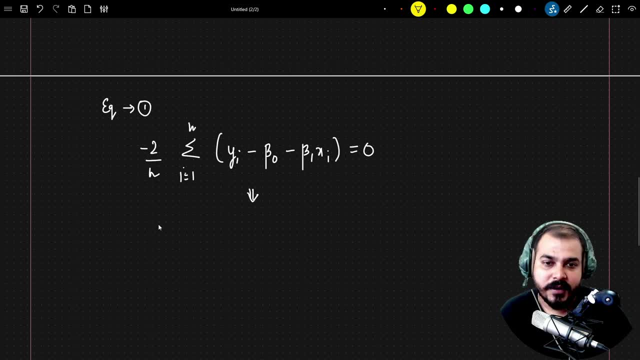 So here in this equation I can also write something like this. I will now write: summation of i is equal to one to n, and this will be minus over here, y of i minus beta zero, minus beta one x one. Okay, 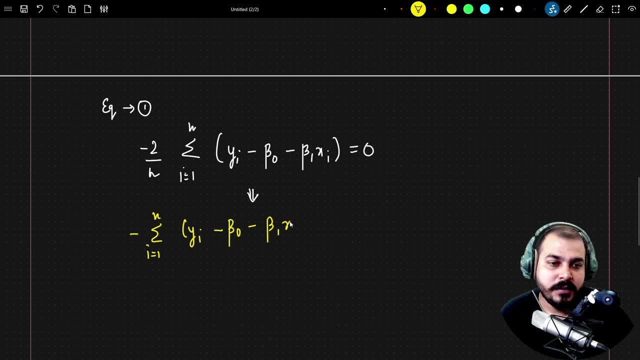 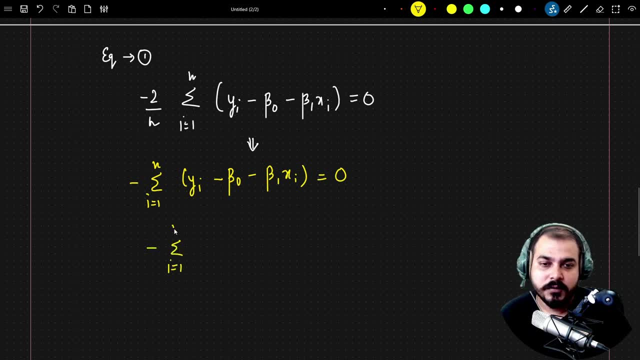 i right. So now here you'll be able to see I will be getting minus. submission of i is equal to one to n. y of i, This will be plus, Since I don't have any variable that is ranging between one to n. so here I can directly multiply. 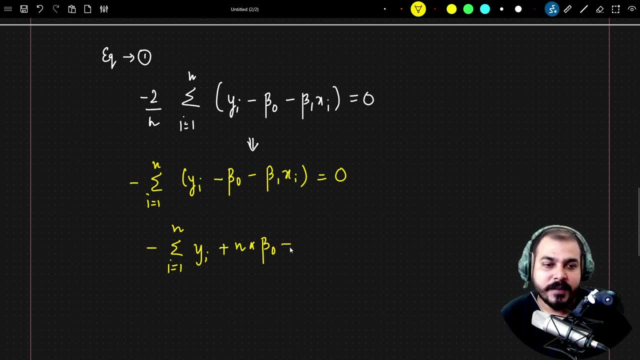 n multiplied by beta, zero, minus, And again this minus a will equal one to n, because we have zero here, which was two. Minus into minus will be plus, And here you know that I can write: beta 1, summation of i is equal to 1 to n. x of i is equal to 0.. 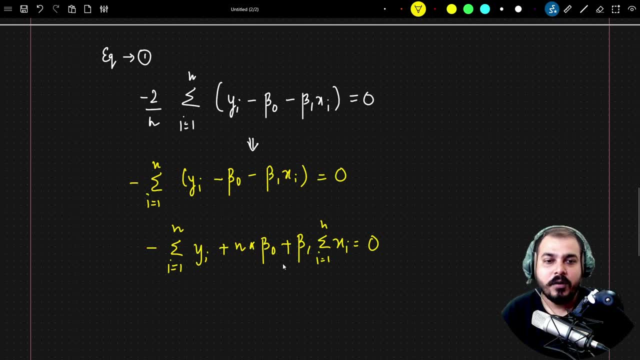 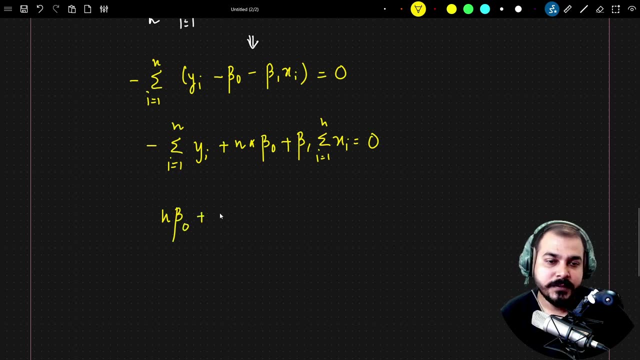 Okay, So this is what we have actually done over here. Now all I have to do is that I can basically consider: n multiplied by beta 0 plus beta 1, multiplied by summation of i is equal to 1 to n, x of i is equal to. I will move this entire equation over here. 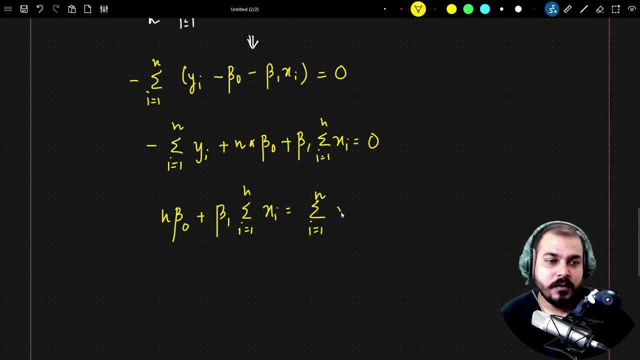 So this will become: summation of i is equal to 1 to n y of i. Okay, Now again, my aim is basically to calculate beta 0.. Let's say, from this I'll be writing, beta 0 is equal to: now here you have. summation of i is equal to 1 to n y of i minus. if I take this value over here, that will be beta 1. summation of i is equal to 1 to n x of i. 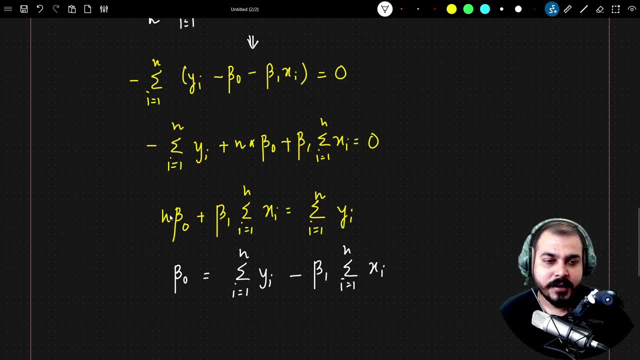 Okay, And here you already know that I have n, Now n. what I'm actually going to do over here, I'm going to, I'm going to move it in the below denominator. So let's say this is also divided by n, and this is also divided by n. 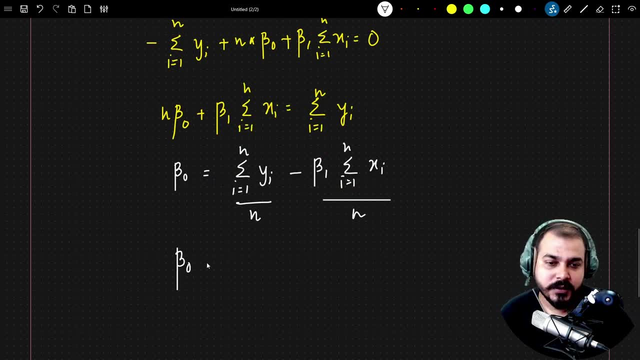 Okay, So finally I can prove that my beta 0 is nothing. but if what is happening over here, see, this is nothing. but this is the summation of y of i divided by n. So this can I say: this is the average. 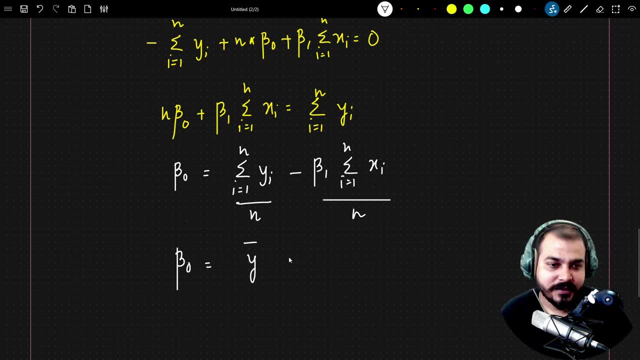 So definitely I can write this as y of y. hat right, So this becomes an average. And similarly over here: x of i. summation of i is equal to 1 to n. x of i divided by n. This is nothing but beta 1 multiplied by x bar. 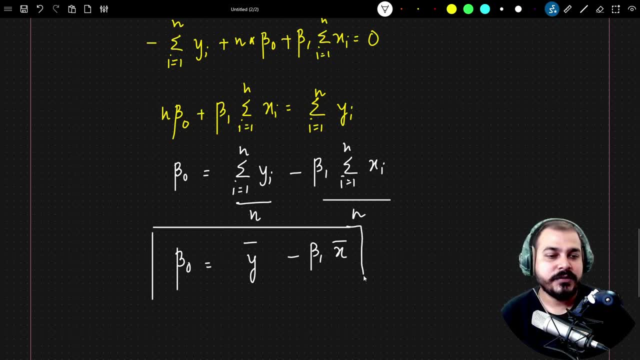 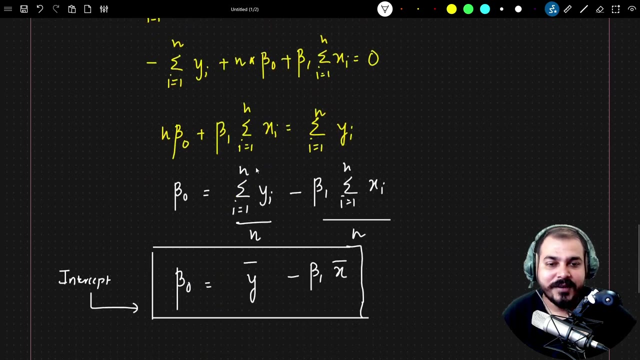 So beta 0 in this entire equation can be calculated by using this particular equation, Right? So my intercept, if I really want to calculate my intercept, my intercept can be calculated by using this. Okay, So just imagine we have taken the first equation from here after doing the derivative, and we have computed how to calculate beta 0. 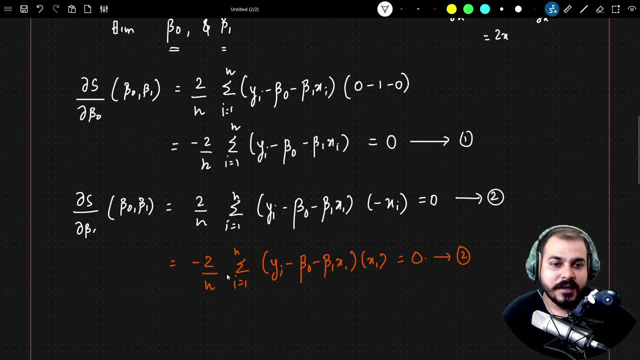 Now let's take the second equation and let's do the same thing. Right Now. in the second equation, you know that it is minus 2 by n, So here what I'm going to do, let's consider equation 2.. 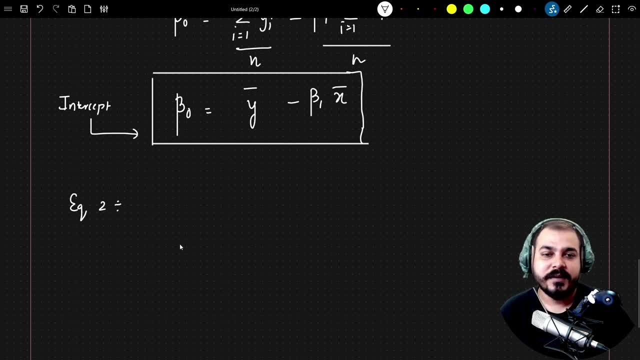 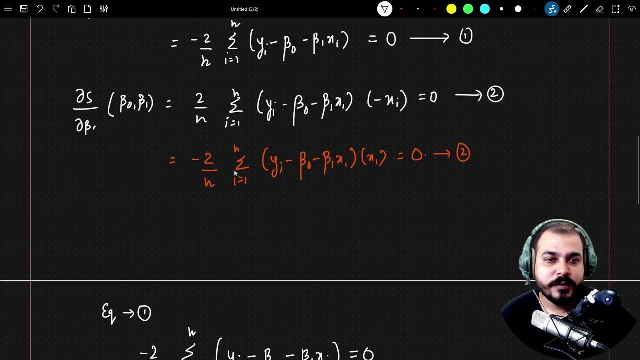 Let's consider equation 2.. Now, since we have got beta 0 over here, obviously now it will become easy to get the beta 1, right, And beta 0 is nothing, but it is the intercept. Now equation 2,. I'm just going to write minus 2 by n. 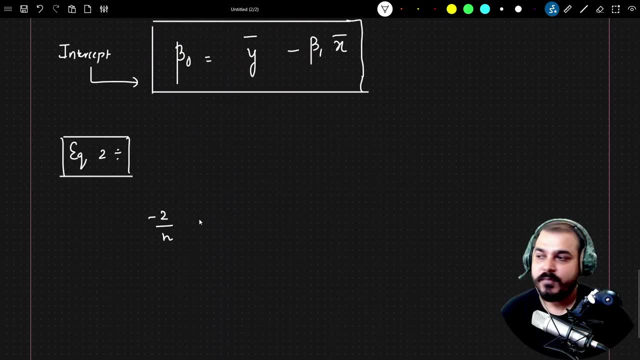 So let's go ahead and write over here. minus 2 by n, And here I'm just going to write it down from my notes: i is equal to 1 to n. y of i minus beta, 0 minus beta 1.. x of i multiplied by x of i right is equal to 0, right. 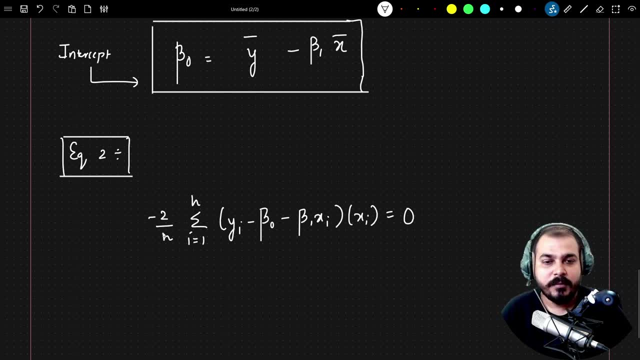 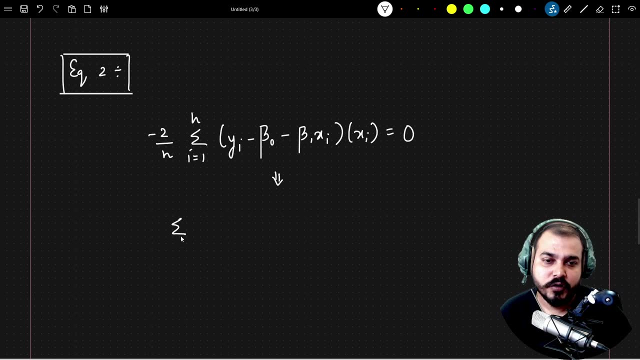 So this is the equation that I actually have Now. this 2 will go to the denominator, n will go to the numerator, So everything will become 0.. So now I can write this equation as again same thing. here I'm just going to write: summation of i is equal to 1 to n, y of i minus beta 0, beta 1, x of i multiplied by x of i, which is equal to 0. 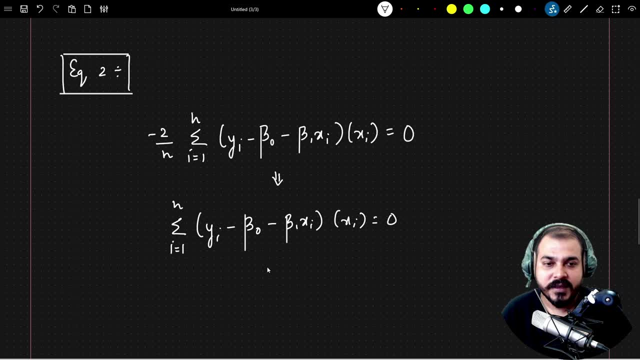 Okay, And the next thing that we are probably going to do Okay Over here is that let's multiply x of i and summation of i is equal to 1 to n inside this. Okay, So after we multiply this here, you'll be able to see I'll be getting summation of i is equal to 1 to n. x of i multiplied by y of i. 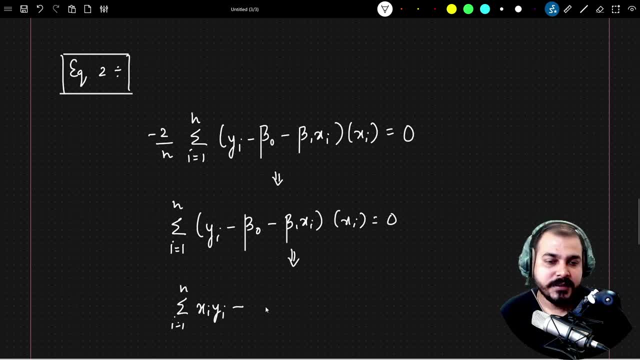 So this will be x, i, y, i, And then I will get minus beta 0, summation of i is equal to 1 to n And this x of i will get multiplied over here And minus. here you'll be seeing I'll be getting. 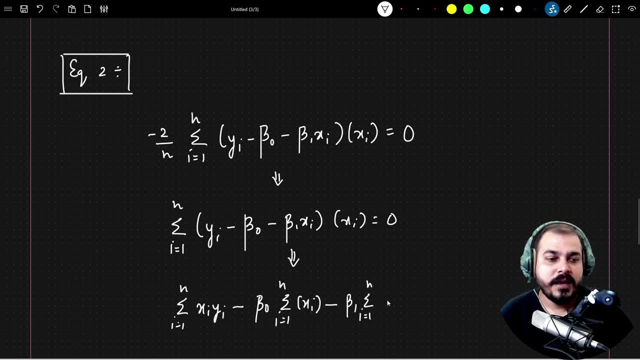 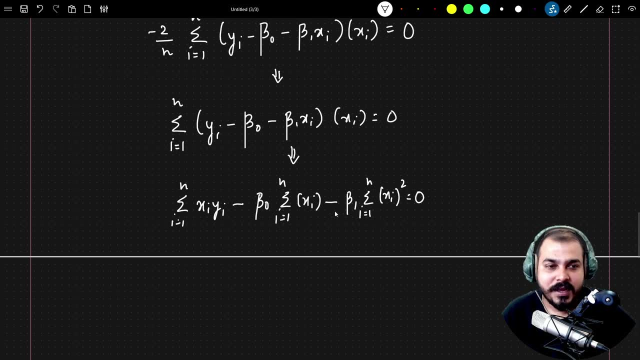 Beta 1, summation of i is equal to 1 to n, and this will be x of i. whole square, Right. So this is the equation that will happen after doing all these things. Now, one common thing that you see is: summation of i is equal to 1 to n. 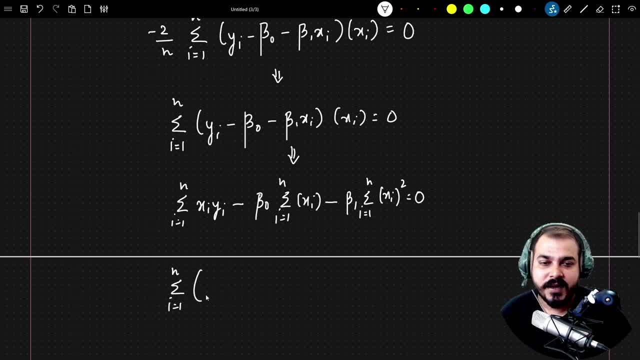 So what I can do, I can take it as summation of i is equal to 1 to n, Then this will become x of i, y of i And this will be beta 0 of x of i And this will be beta 1 into x of i whole square. 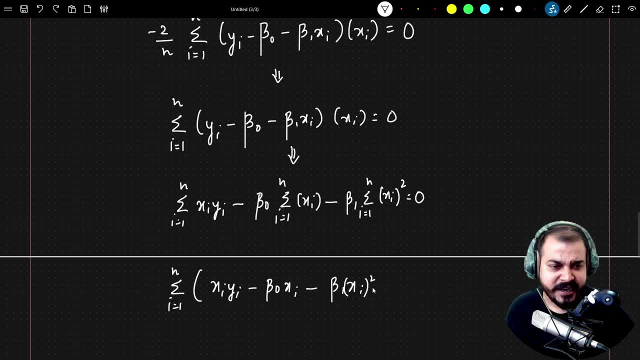 Right, And this will be. Let me write like this: Beta 1, x of i whole square And this will be basically equal to 0.. Now you know that beta 0 value. you already know It is y hat minus beta 1 into x bar. 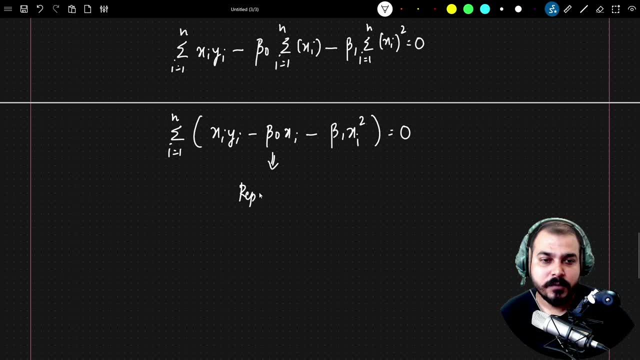 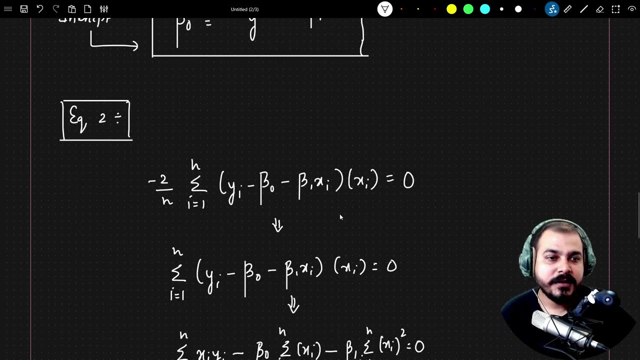 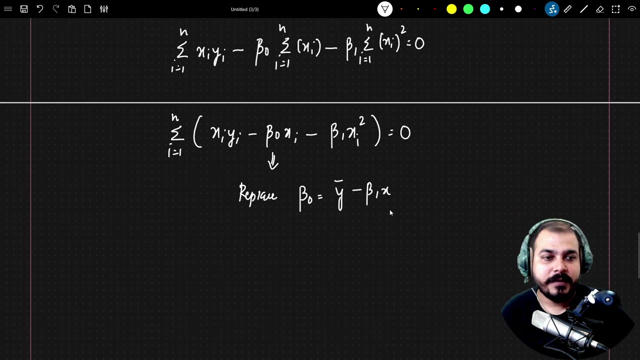 So what I'm going to do, I'm going to replace beta 0. With y hat minus y, hat minus beta 1 into x. So if I replace This into this beta 1 into x bar, right then what will now happen? 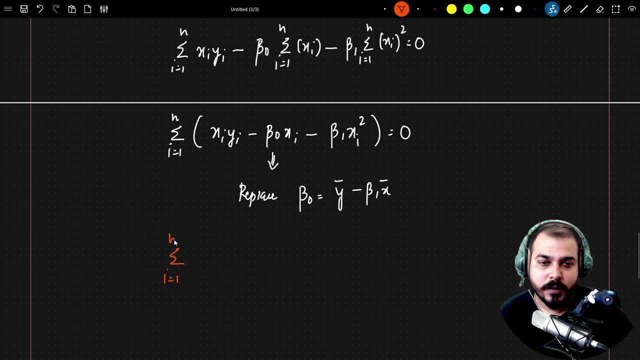 Now let me go ahead and write in different colors, So this will be summation of: i is equal to 1 to n. X of i. y of i minus beta 0 is nothing but y hat minus beta 1 into x bar. 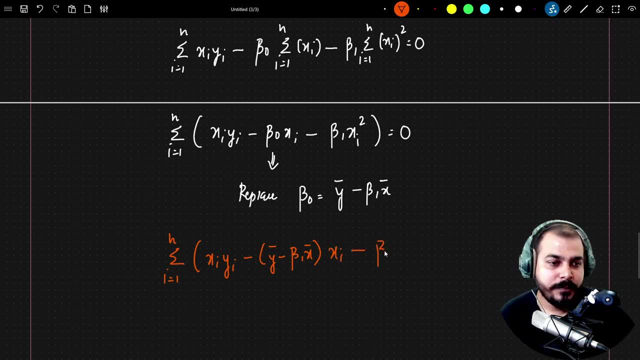 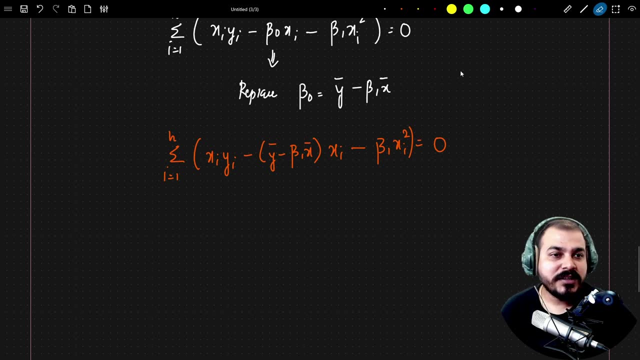 And then you have x of i minus beta 1, x 1, x of i whole square, And this is basically equal to 0.. So, guys, now, once we replace beta 0 by y bar minus beta 1 into x bar, Here you'll be able to see this: 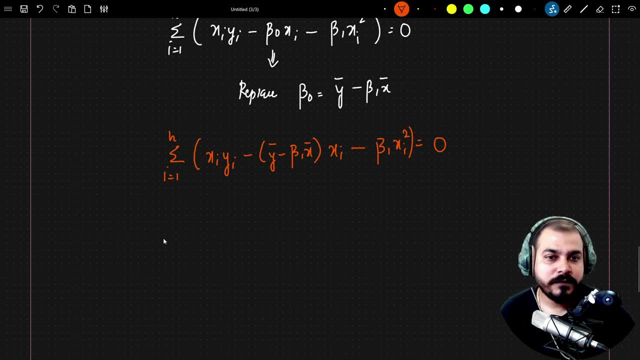 Now, in the next step, what I will do. I will just write: summation of I is equal to 1 to n and I will be multiplying x of i inside this. OK, so this will be x of i- y of i minus x of i- y- bar. 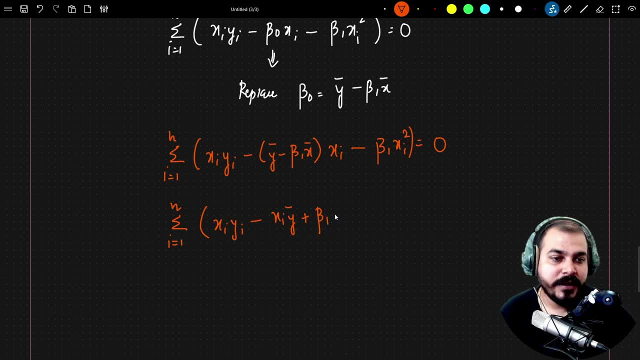 Then this minus into minus will be plus. Then here I can write: beta 1: x, bar x of i minus beta 1. X of i- whole square. Now you will be knowing why we are doing all these things, because at the end of the day, 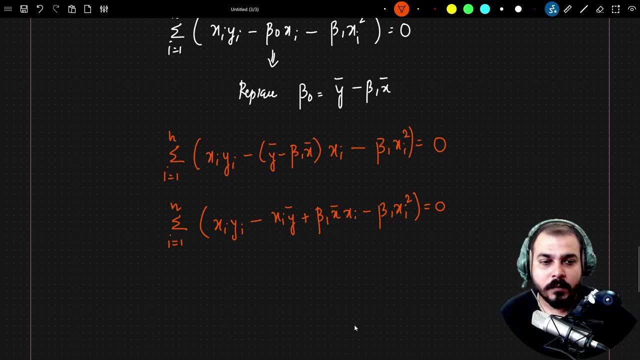 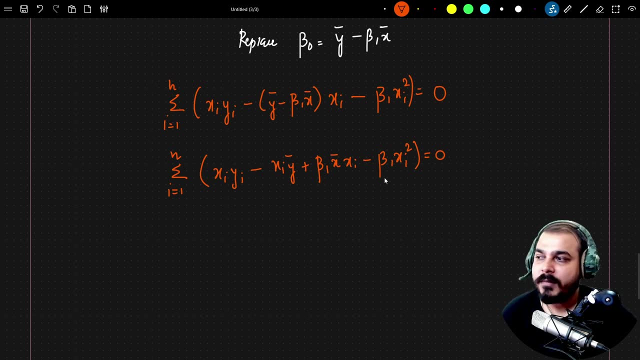 we'll be getting an equation to find out beta 1.. OK, now the next step after this. what we basically do is that here in all this equation, the most common thing that you'll be finding is x of i. So let me remove x of i outside. 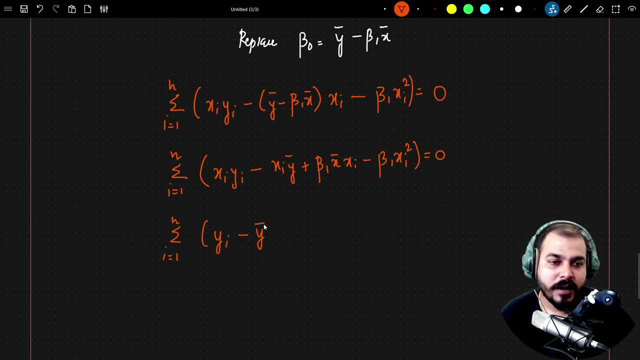 So here we'll basically have y of i minus y bar plus beta 1, into x bar minus beta 1.. into x of i, and this x of i will come outside. OK, now what we do. you can remove this x of i by just putting this in the denominator: 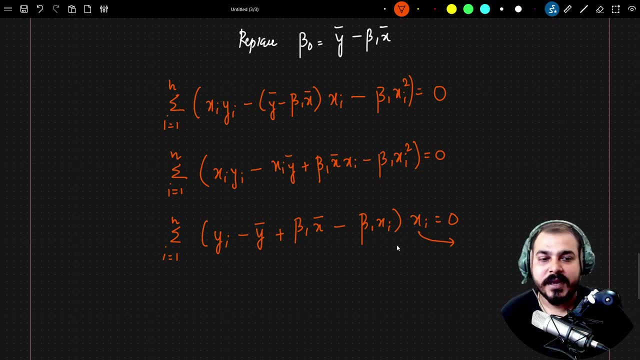 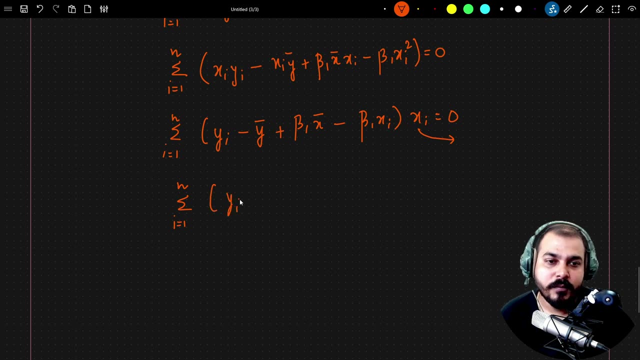 So obviously this will be entirely zero. only this side and this x of i can also be lost. Now the next thing that we are going to do: I will write: summation of i is equal to 1 to n, And here I will write y of i minus y bar. 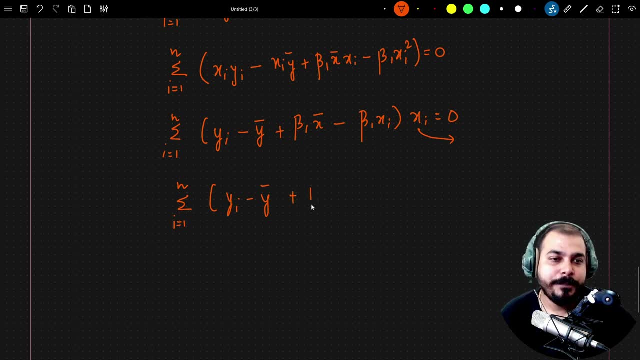 OK, so this is my first equation, And then I will also say beta 1.. And what I'll do here? I will write: x bar minus x of i is equal to zero. OK, finally, now the next step that we are going to do. 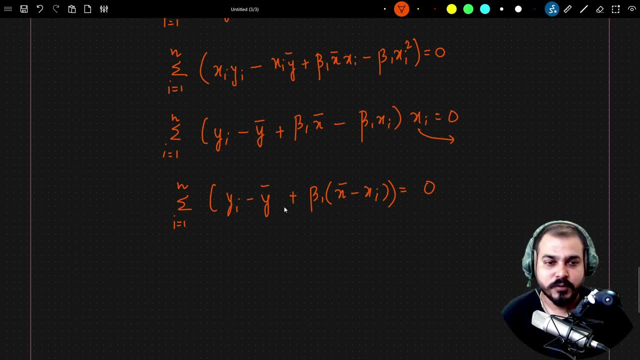 and obviously I can also take this as a separate group- y of i minus y bar together, right? We can also take this like this together, right? Because, understand, I'm just grouping this and I'm taking a common of beta 1 and I'm basically writing: beta 1, x bar minus x. 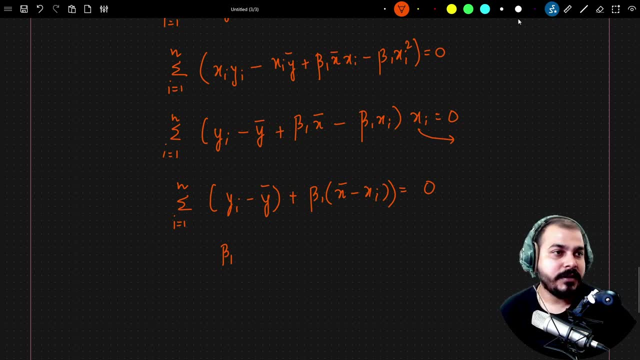 Now what I'm going to do here. I'll write beta 1.. Let's say that this is there. Let's say that this is there. They're outside, in my complete bracket. Now, if I try to multiply the summation of i1, then it will be: summation of i is equal to 1, y of i minus y bar. 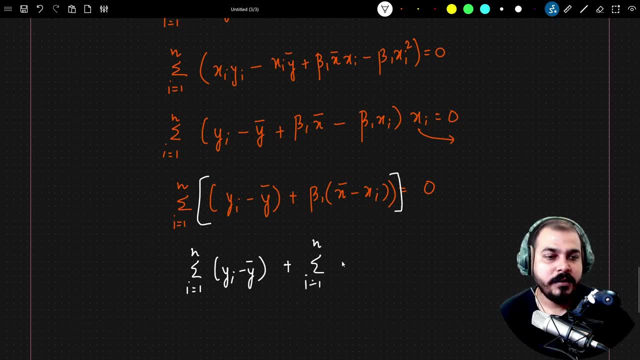 OK, plus summation of i is equal to 1 to n, beta 1 x bar minus x of i. OK, so this is what I'm actually going to get with respect to zero. OK, so I've just made it into two groups. 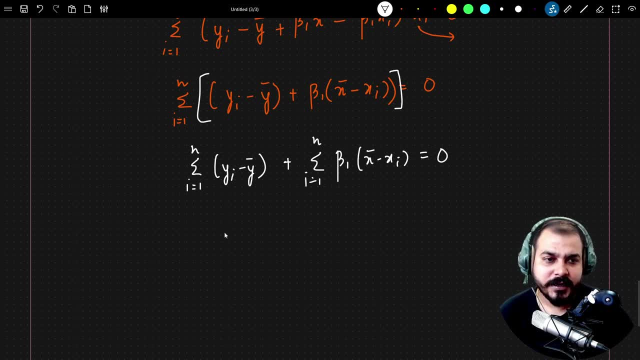 OK, now, after this, I can definitely write something like this: Summation of i is equal to 1 to n beta, 1 x bar minus x of i, And here I'm just going to take this as minus, and this will be. summation of i is equal to 1 to n y of i minus y bar. 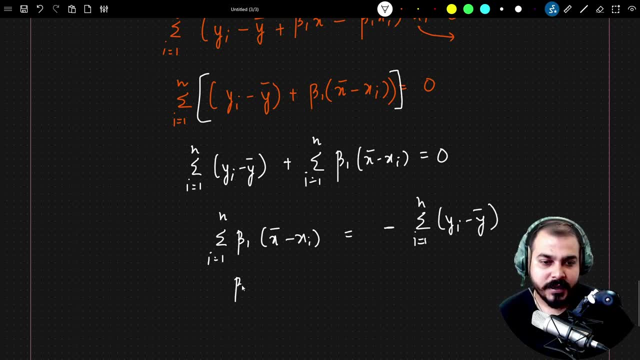 I'm just taking this particular equation at this side. Then, finally, I will be getting beta 1, which will nothing be. It will be minus. summation of i is equal to 1 to n. OK, y of i minus y bar. 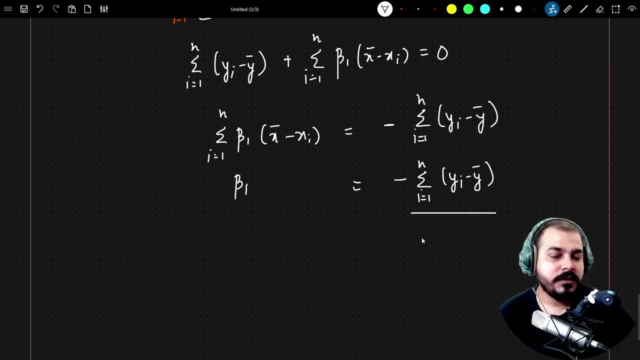 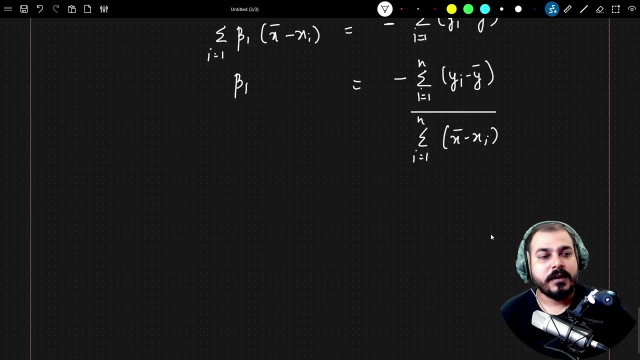 OK, Y of i minus y bar, divided by summation of i, is equal to 1 to n And this will be x bar minus x of i. Now see over here: if I try to bring this x of i forward, then I have to probably take a negative value. 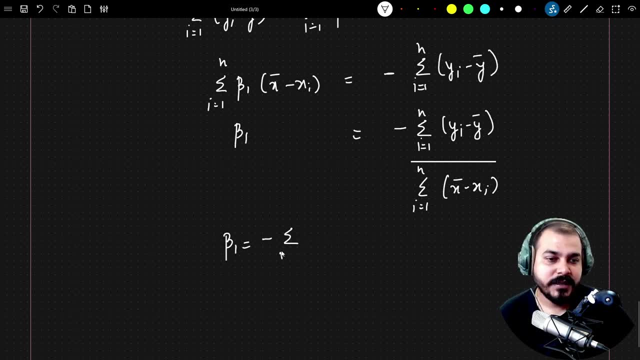 So here, finally, you'll be seeing that beta 1, I can write it as minus, i is equal to 1 to n, y of i minus y bar, And if I take a minus value outside, then I can also write this as i is equal to 1 to n. 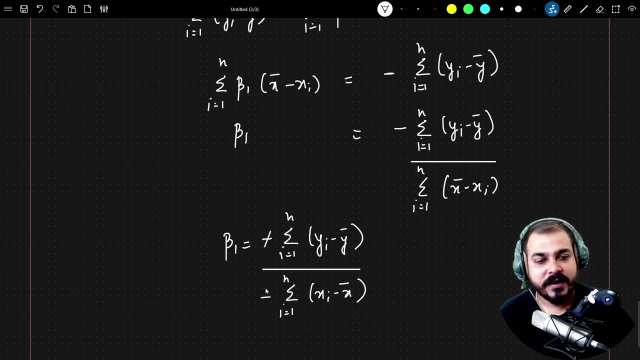 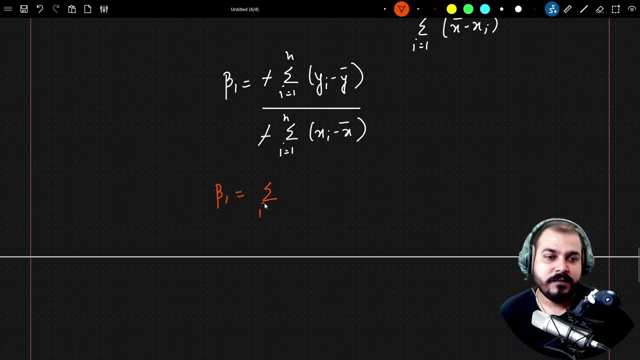 And x of i minus x bar right. This minus and minus will get cancelled And finally, my equation of beta 1 will be: summation of i is equal to 1 to n. y of i minus y hat. divided by, summation of i is equal to 1 to n. x of i minus x bar right. 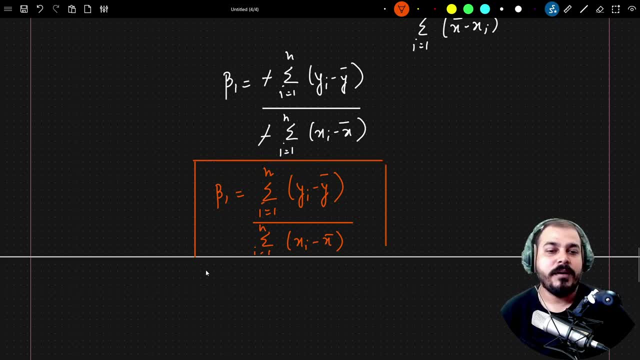 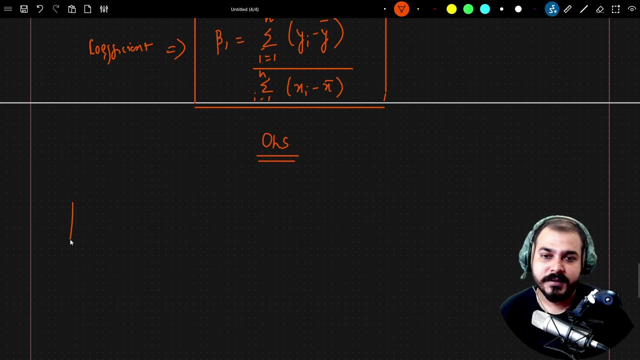 So this is my entire equation of calculating beta 1.. And, if you remember, beta 1 is nothing but It is the intercept, So sorry, it is the coefficient. So, finally, I have actually proved you that with the help of OLS, if you really want to calculate the beta 0, then your formula is basically given over here, which I've actually proved it. 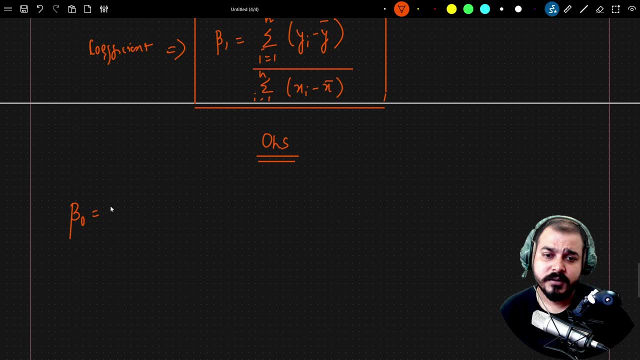 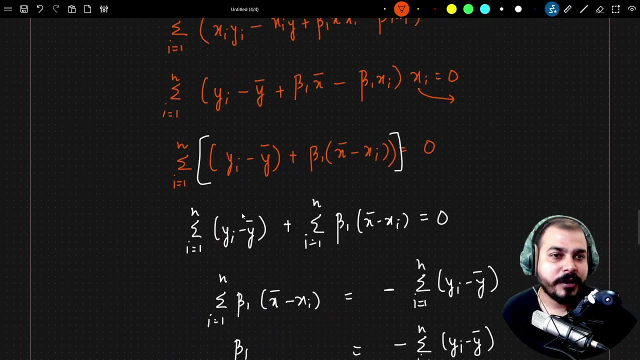 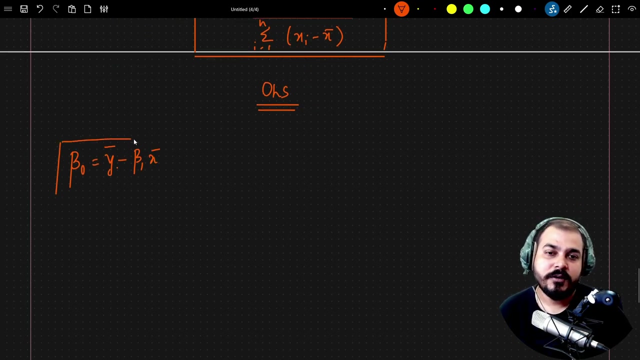 Y hat minus beta 1 into x bar. So here you'll be seeing: y hat minus beta 1.. I think beta 1,. right Now let me write a beta 1 into x bar. right, X bar. This equation is basically to calculate the intercept. 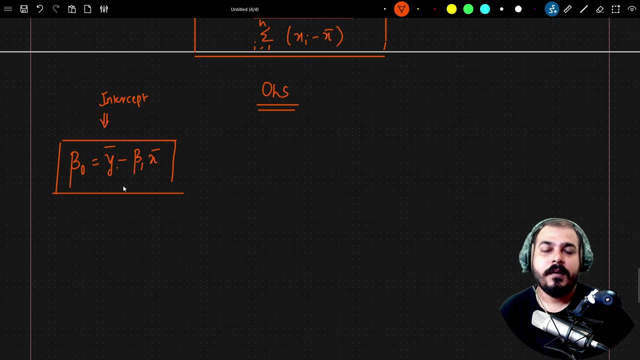 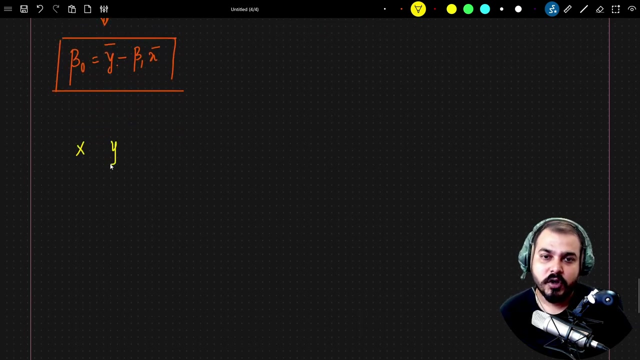 This equation is basically to calculate the intercept, And in order to calculate the coefficient we use this specific equation, that is, y of i minus y bar, divided by x of i minus x bar. So let's say I have some data points- x, comma, y- and here you'll be having some values. 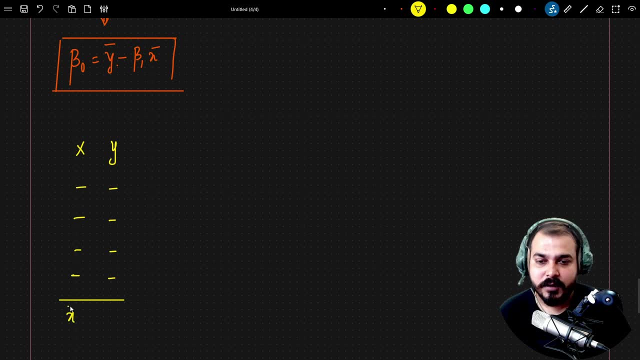 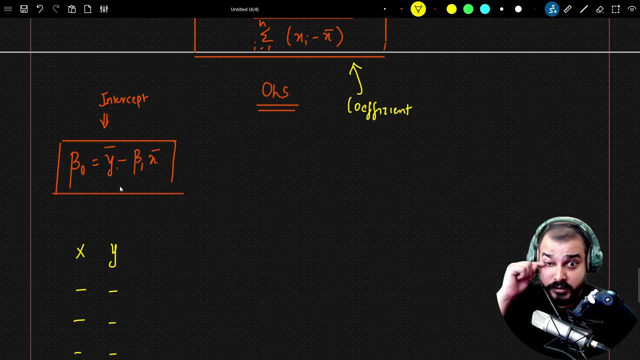 Okay, From this, obviously, you'll be able to calculate x bar and y bar, And all you have to do in order to calculate beta 0, you just have to equate this particular equation, y bar minus beta 1, into x. 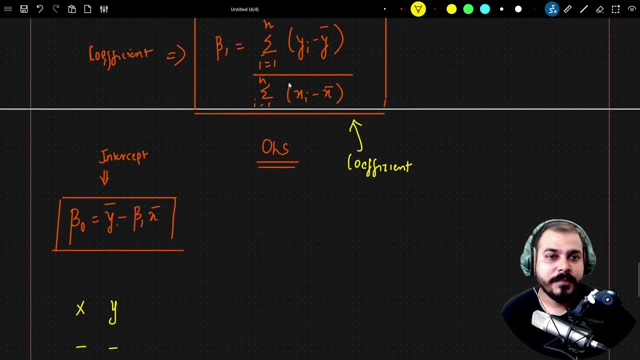 First of all, if you really want to calculate beta 1, first of all, we'll go ahead and calculate beta 1 over here And beta 1, you know, y of i, y hat, So you'll go and compute this component. 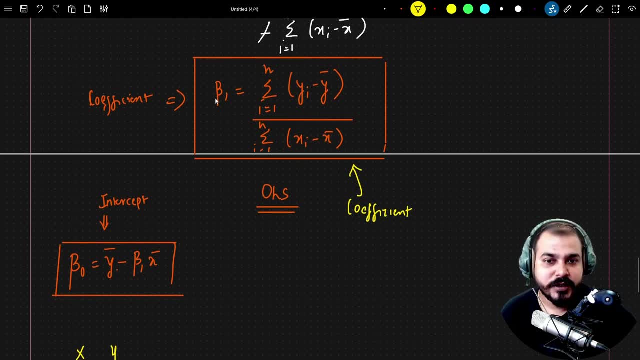 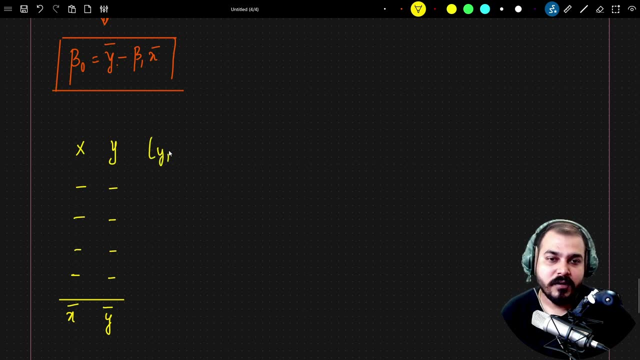 You'll go ahead and compute this component and you'll divide this both. You'll get beta 1.. Once you get beta 1, you can equate this over here, right? So first thing, let's see over here: You'll calculate y of i minus y bar, right. 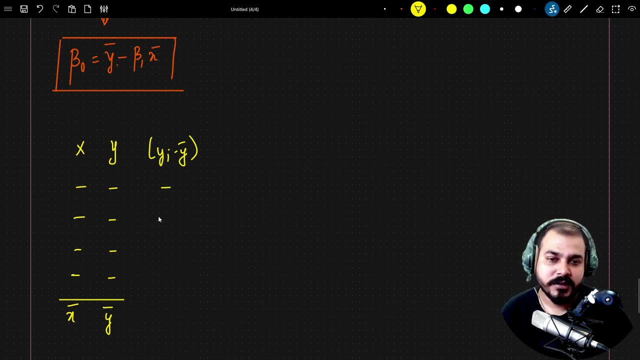 With respect to every point. you know, whatever y bar is there, you'll get all these values right And then you'll calculate x, i minus x bar. Here you'll be getting all the values. Then you divide in both of them. 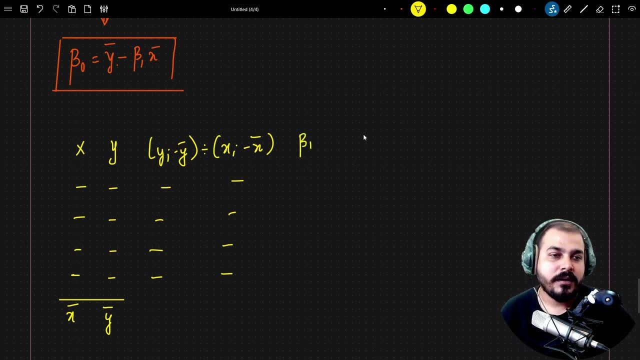 Once you divide in both of them, you'll basically be getting beta 1.. And after that you can equate in this particular equation beta 0 equal to y hat minus beta 1 into x bar. Then you'll be able.